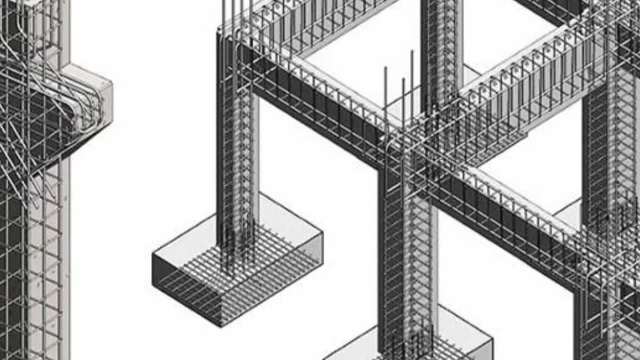 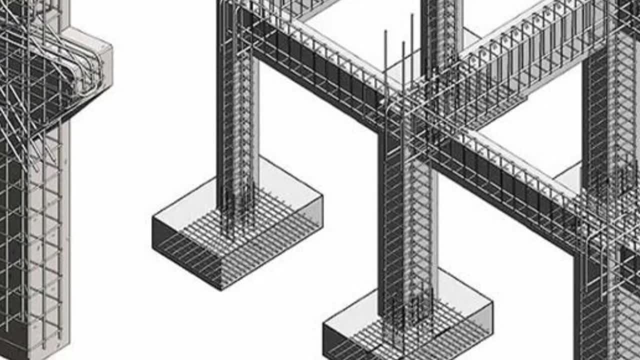 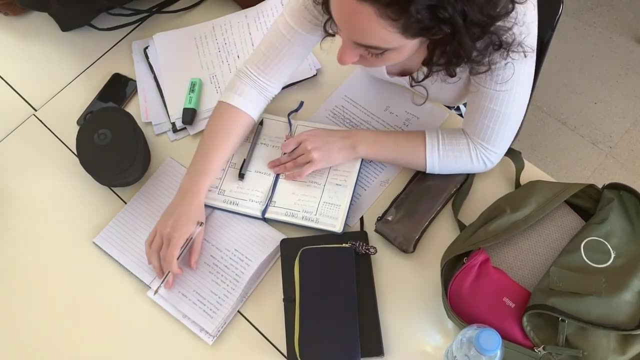 design project, we also start by analyzing our beam elements. We transfer wall and slab load to columns and from columns to foundations. This analysis and cross-checking processes are tedious and time-consuming when verifying our results by hand. Hence, for those of us 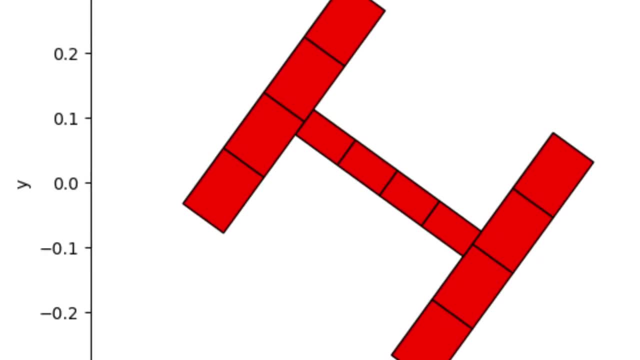 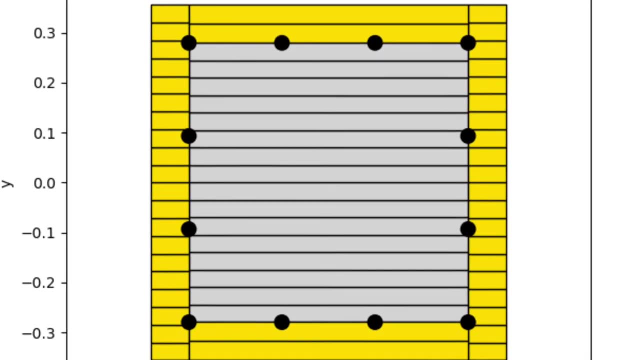 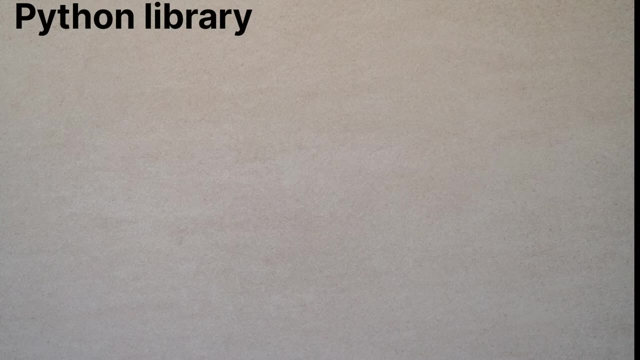 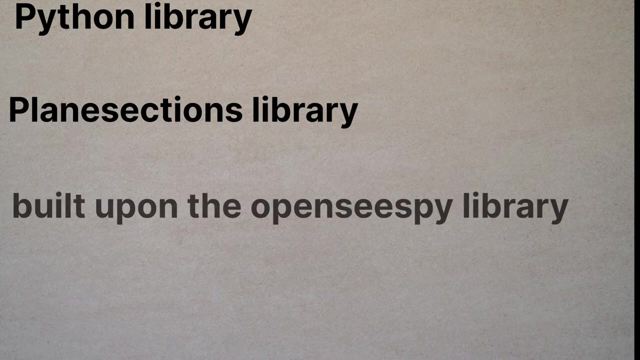 with interest in developing finite element tools for structural analysis. this is going to show us how to create a simple beam model and plot its shear force and bending moment diagram using a Python lightweight library called PlaneSections. This library is created by CS Bloom, which is built upon OpenSees. 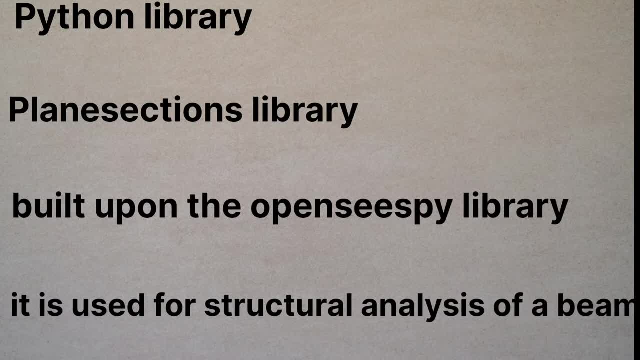 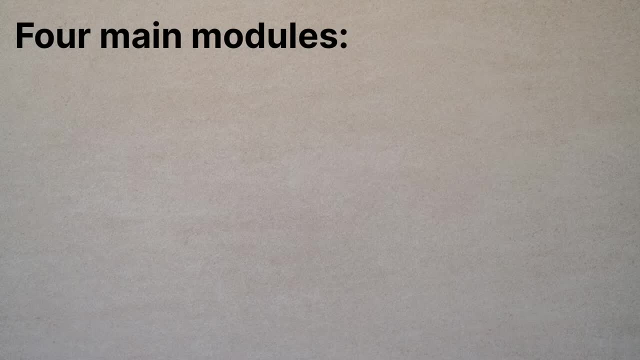 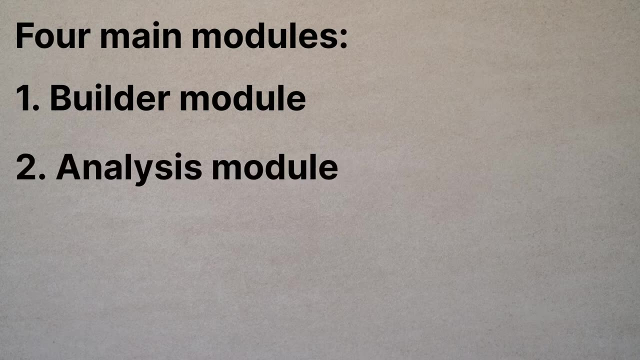 Py. So this PlaneSection library has four core models which you have to understand. The first is the Builder module, which is used to create the beam and beam element. The second is the Analysis module, which is used to analyze the beam using OpenSees Py. 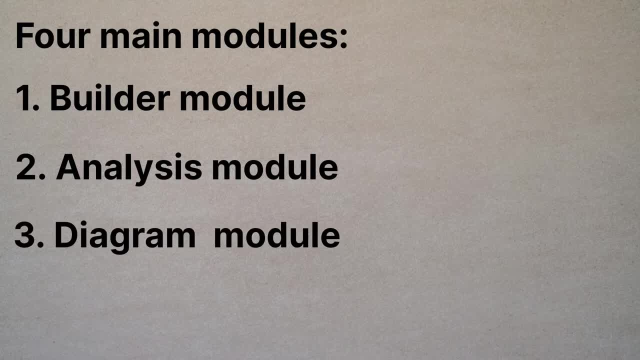 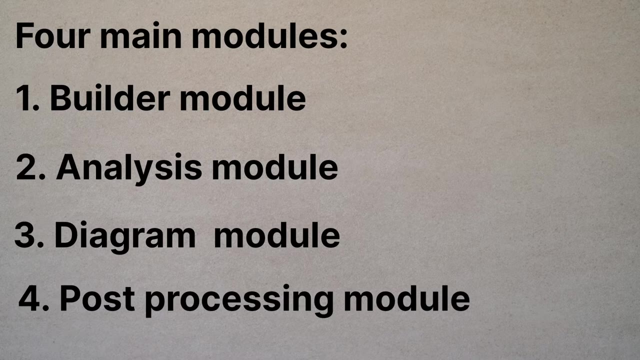 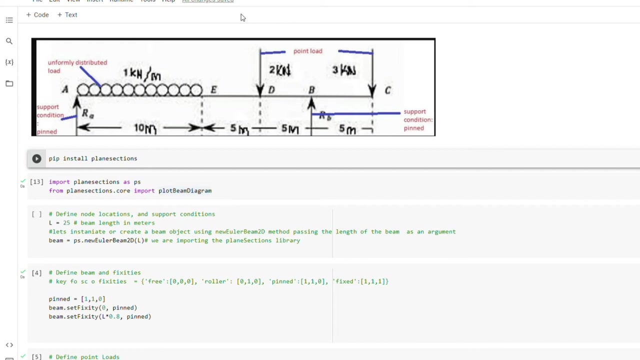 and document the result. The third is the Diagram module, which is used to plot the beam module, And the fourth is the Post-Process module, which is used to plot the response of the beam. Okay, this is the beam we are going to be modeling and plotting its shear force and bending moment diagram. 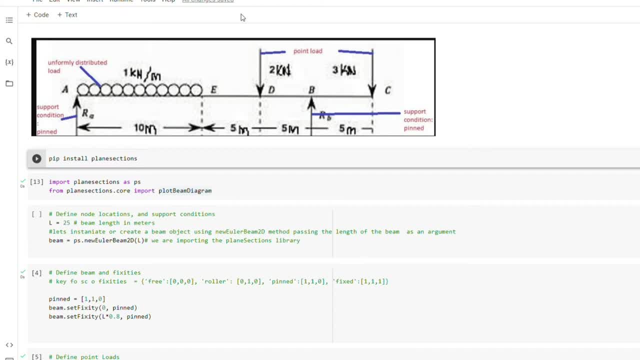 So, as you can see, we have a beam spanning up to 25 meters length. We have two support conditions, at A and B. We have uniformly distributed load, which is 1 kilonewton per meter spanning from A to E, which is 10 meters. 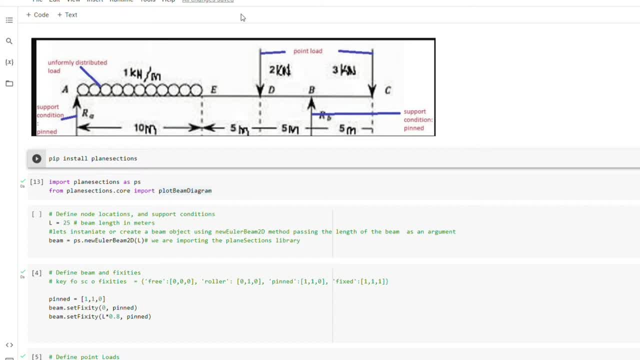 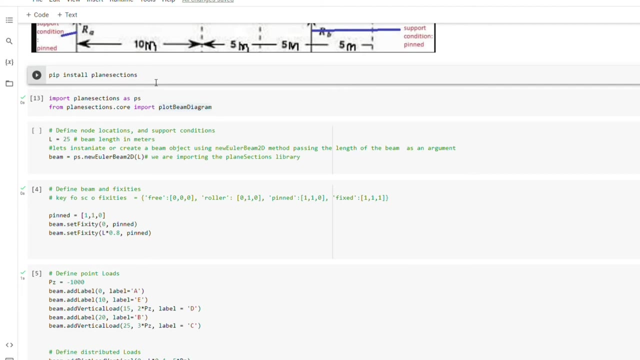 And then we have two point load, which is at D and C, 2 kilonewton and 3 kilonewton respectively. So the first thing we are going to do is to install our plane section library, And this is the command used. 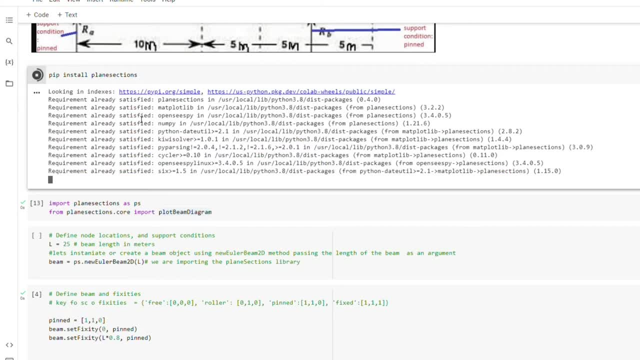 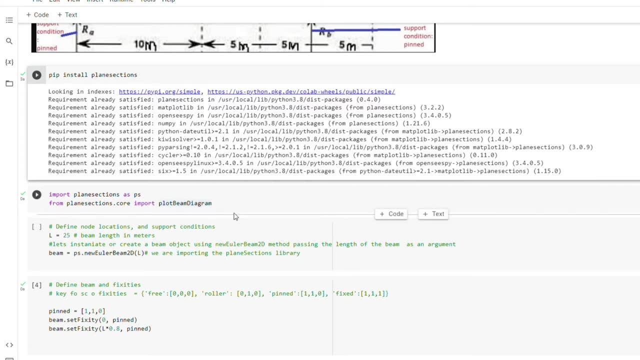 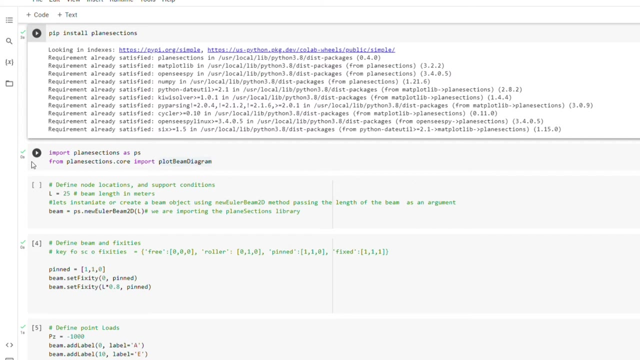 We are using pip- install plane sections- So we are going to run it And I've already installed the library, So maybe you doing it for the first time is going to take some time before it finishes. So the second thing is for us to import the plane sections as PS. 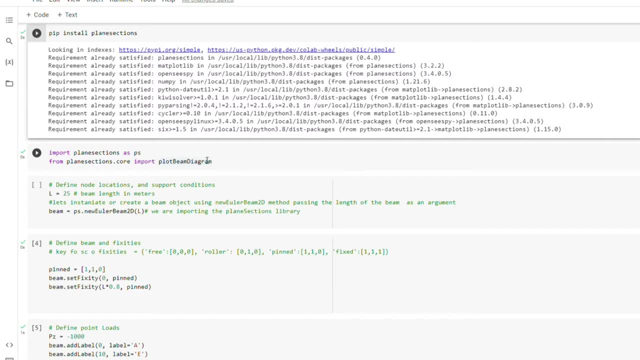 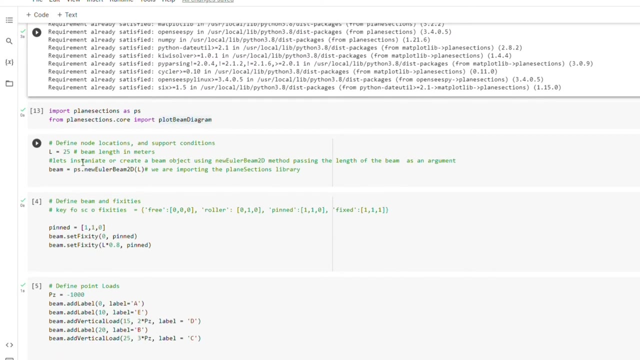 Or you can name it as anything you like, But this is how the convention that I use. So we are also importing The plot diagram class from the plane section dot core. So the next thing is to define the node locations and support conditions. 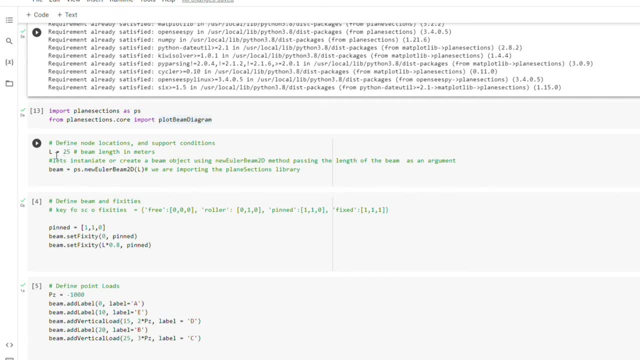 So I define the length of the beam here in a variable which you can see. So we are going to instantiate or create a beam object using the new ELA beam 2D method And we are going to pass the length of our beam that we have created as the argument. 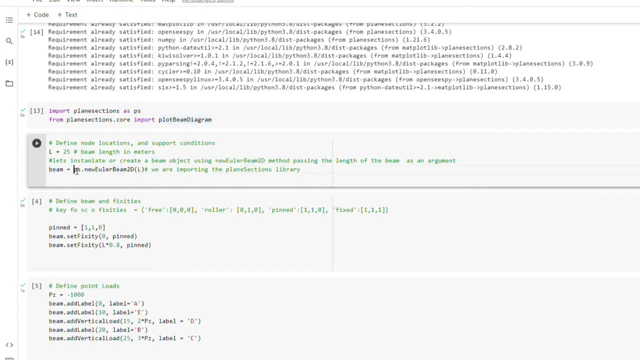 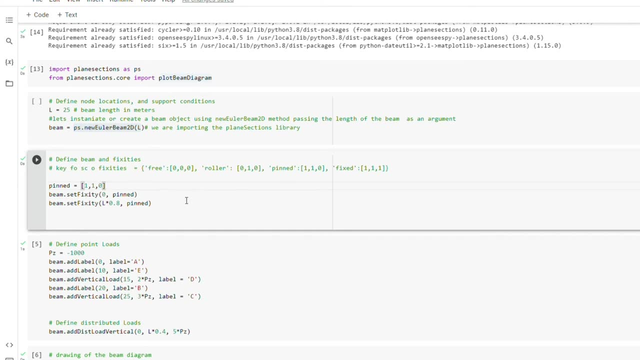 So, as you can see, I've instantiated a beam class here And this is the command. So after that we are going to set fixity or set the or define the support conditions of the beam. So, as you can see, this is like a legend or a map of how you can define different support conditions in plane sections. 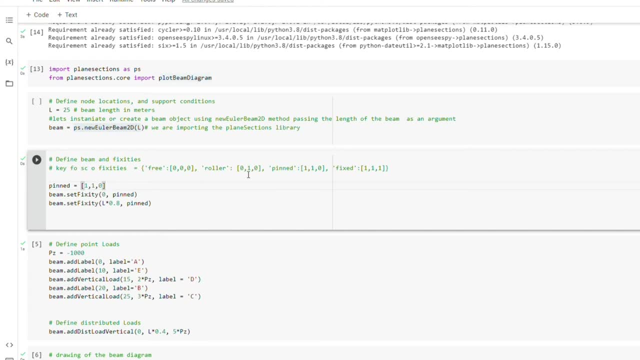 So, as you can see, for free is 0 0 0.. For roller is 0 1 0.. For pin is 1 1 0. And for fix is 1 1 1.. So we are defining pin, since, as you can see from our diagram, 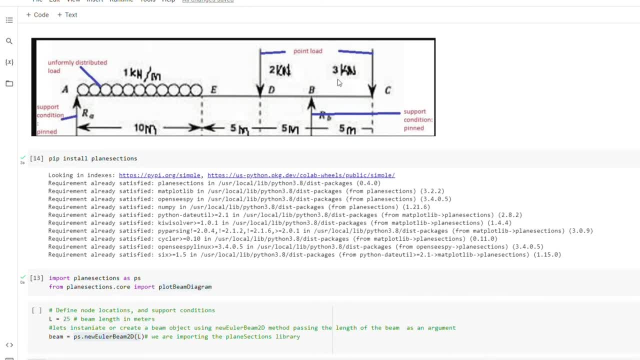 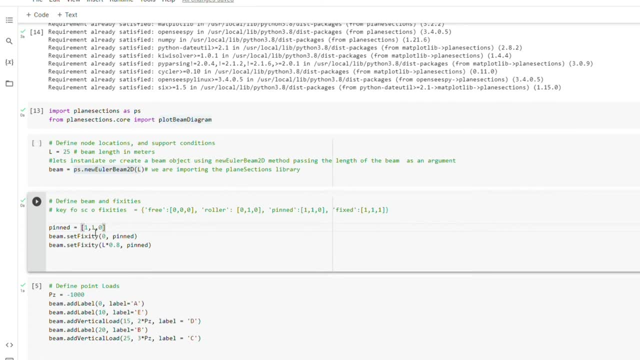 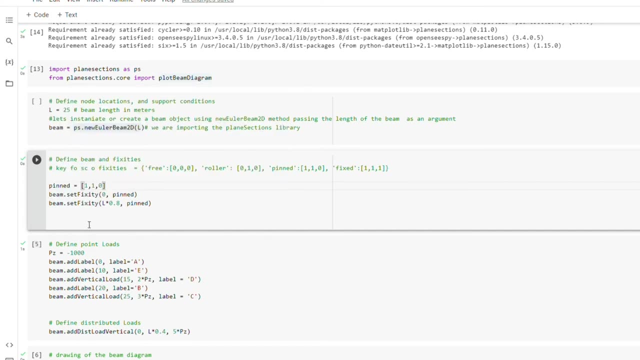 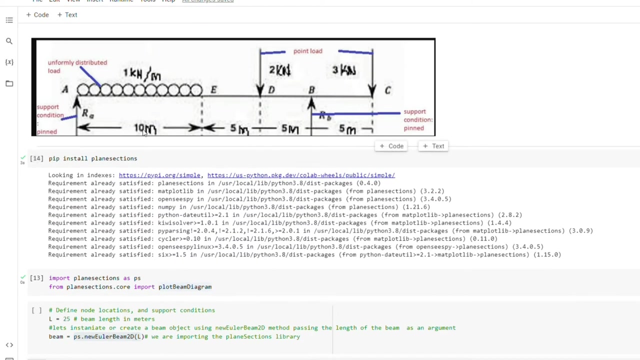 Our support is pin both at A and B. So we are using the 1, 1, 0.. So we are defining the fixity now of the beam from point 0 or distance 0. It's pin. So that is at this position A. 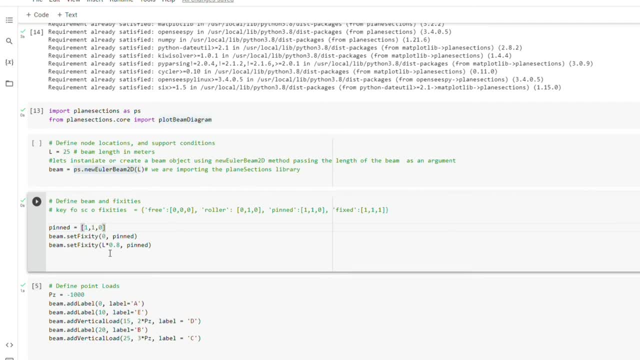 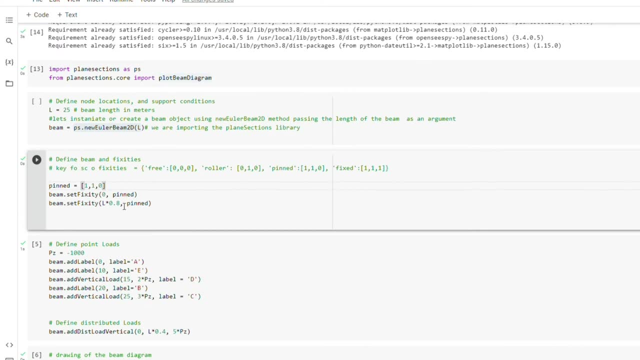 Since the distance here is 0.. So it is pin. And then for the second support condition, that is B, So you can see which is here. So we are multiplying the length, That is, 25 meters, by 0.8, which is going to give you 20 meters. 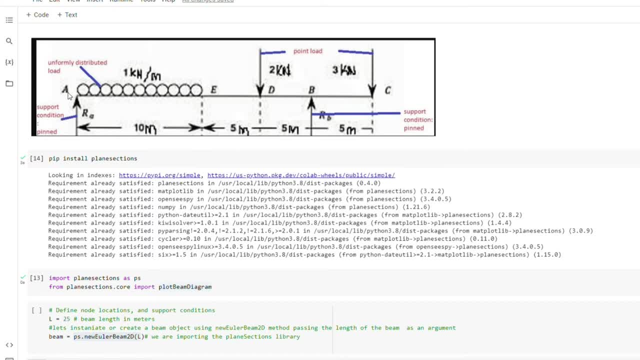 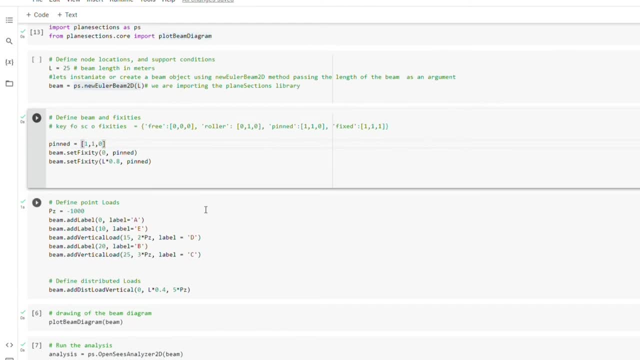 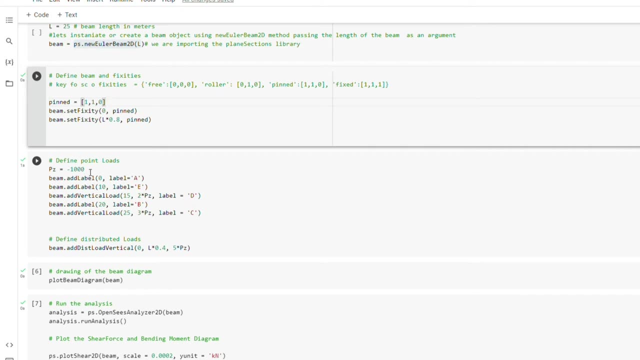 And it is pin also. So when you see from the origin, that is, from A, Which is 10 plus 5 plus 5. Which is 20.. So that is what we did here. So we define our load. So this shows us that the load is acting downward. 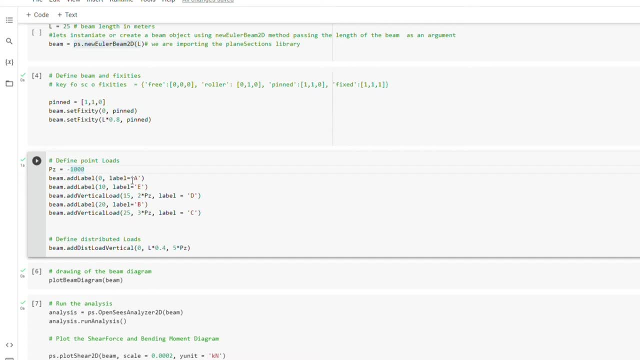 Which is negative, 1000. Or is the same thing as 1 kilo Newton, So beam. So what we are doing here is we are adding the various labels, How the beam was being labeled, So this add label method. We are passing the first argument as the position or the distance. 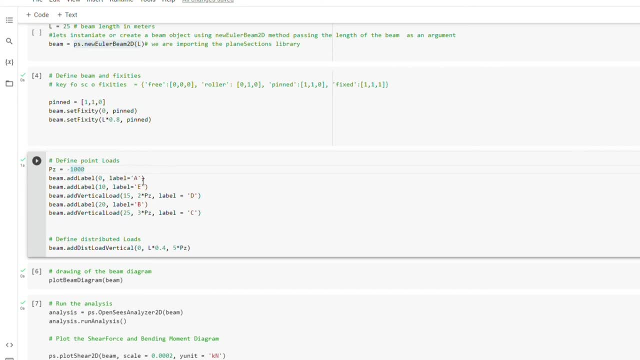 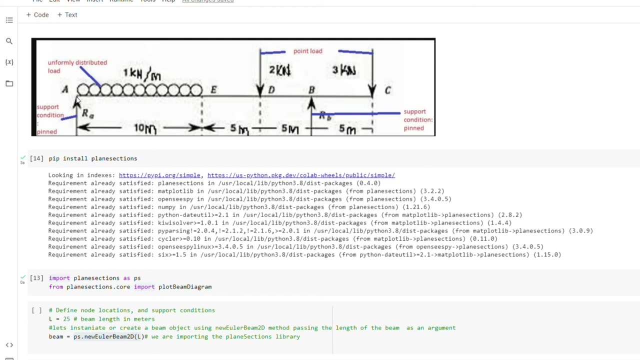 Of where the label is going to be positioned on the beam. So for label A is at position or distance 0. So, as you can see, it is here. Here is the origin, So it is 0. Then, from beam dot, add label. 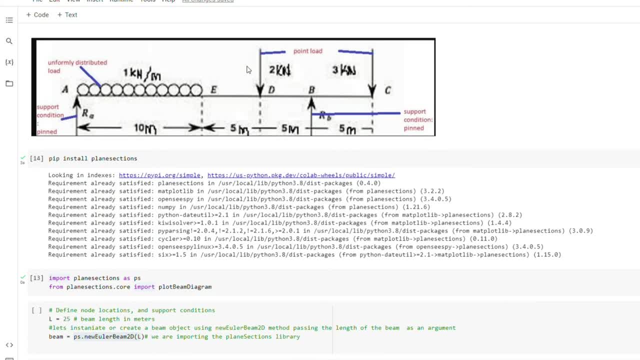 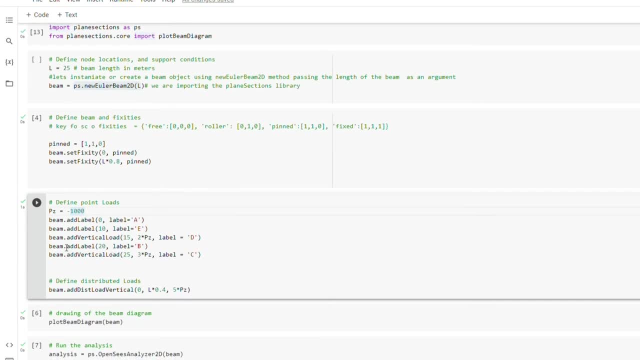 That is the second one. Label E, Which is 10 meters. When you look at E From the origin, that is from A, It is 10 meters. Then for the next thing, we are adding the vertical load. So for the first vertical load, 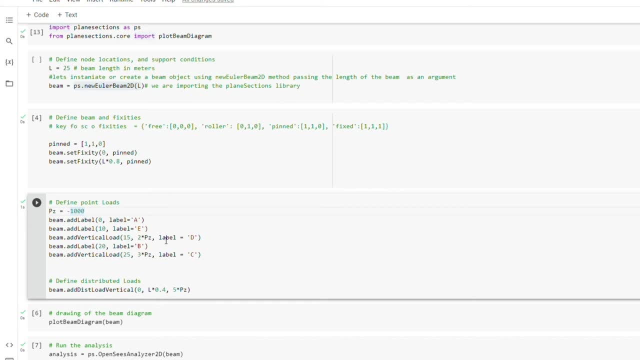 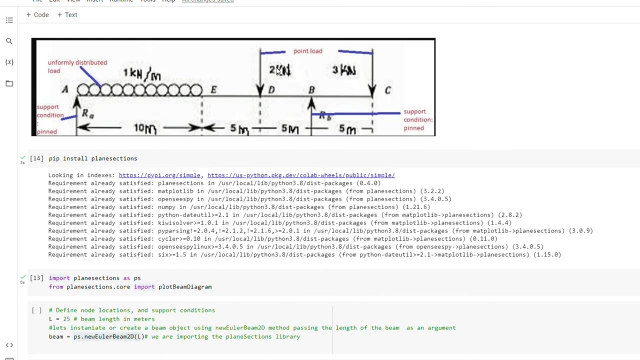 Which is at distance 15 from A. So we have 2 times this load. 2 times this load Which is negative 2000.. Or 2 kilo Newton, And it is positioned at label D. So, as you can see, this is 2 kilo Newton. 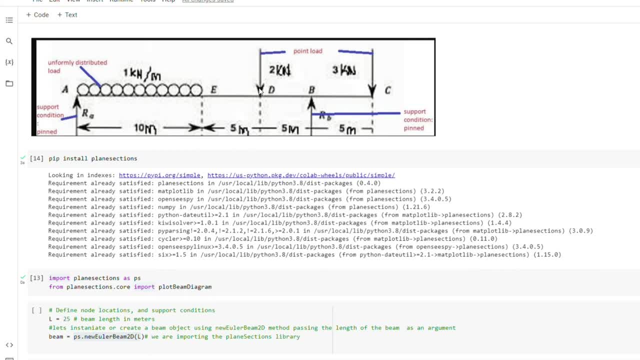 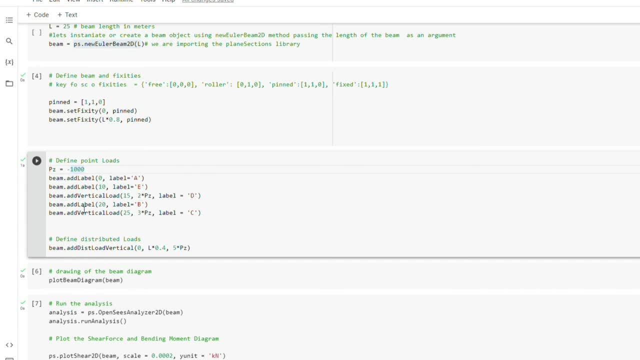 Which is negative, Which, if you can see, the load is acting downward. So then, the next thing is, We are also adding another label, Which is B, And the distance is 20 meters from A Or from the origin. So the next thing is: 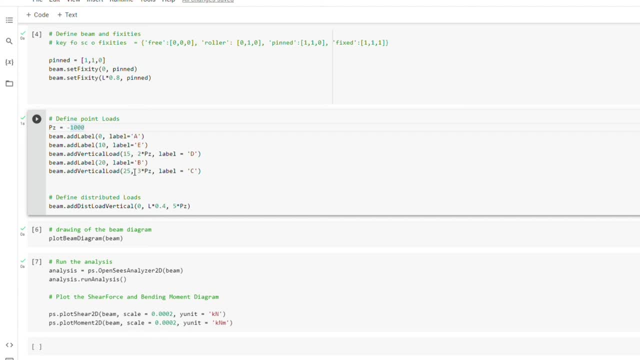 The next thing is: beam dot, add vertical load, Which is 25 meters. That is the position from A, Which we are multiplying this by 3. Which is going to give us 3000. Or 3 kilo Newton, And it is at label C. 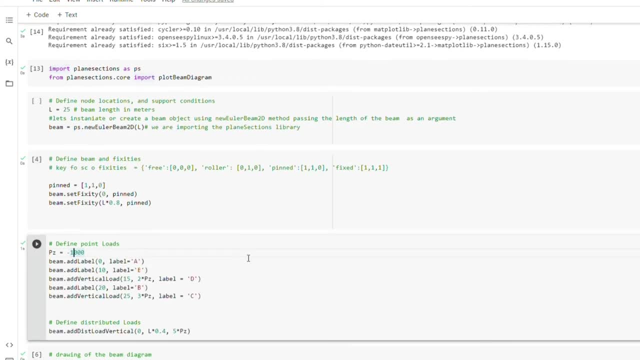 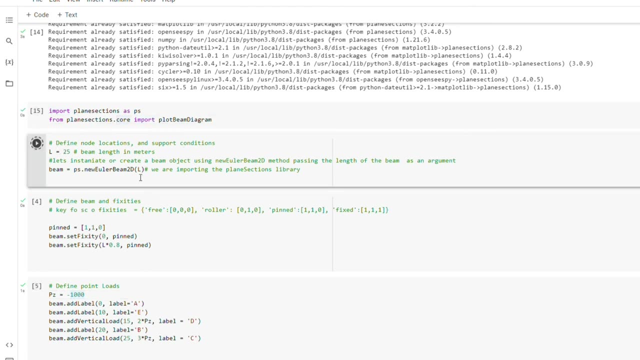 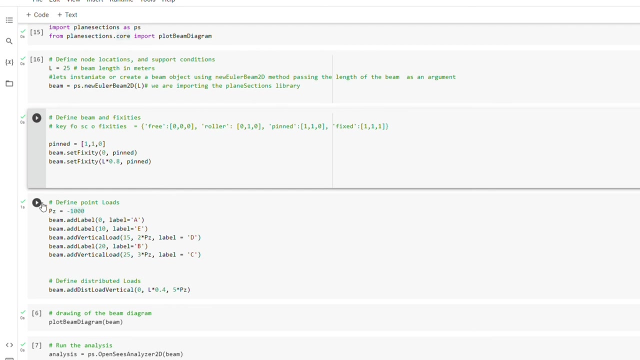 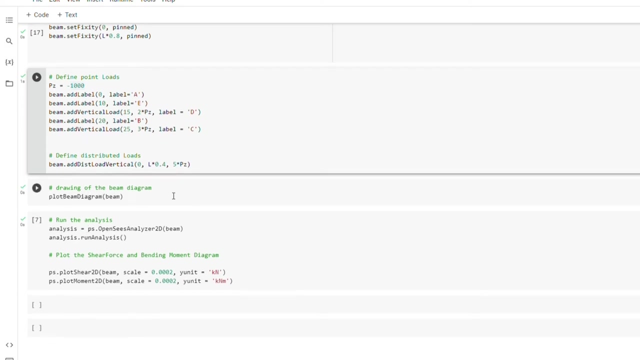 So, as you can see, it is 3 kilo Newton And at label C. So let's run this And let's run this, And let's run this, Then let's run this also. So the next thing is drawing of the beam diagram. 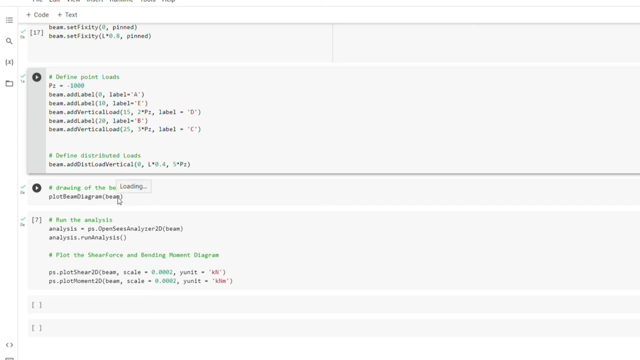 So we are using this plot beam diagram class And we are passing The beam object Because, as you know, we have already created our beam, Giving it all the support conditions And the loadings. So this class is now going to draw our beam diagram. 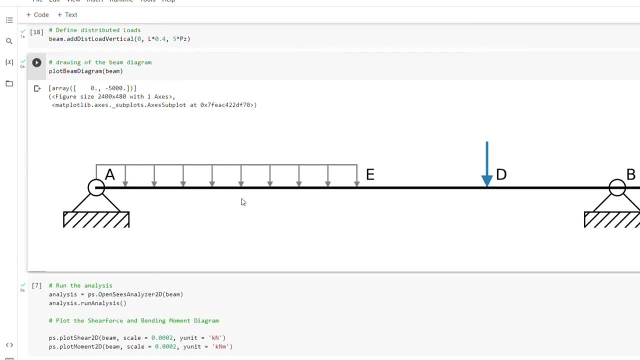 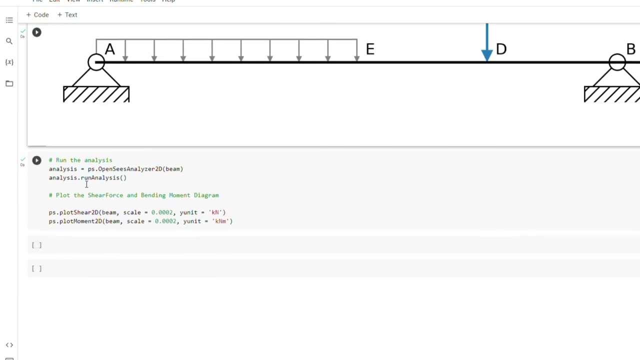 Or our beam model. So let's see, As you can see, We have drawn our beam model with all the loadings And the support conditions. We have drawn this beam And the loadings And the loadings. So the next thing. 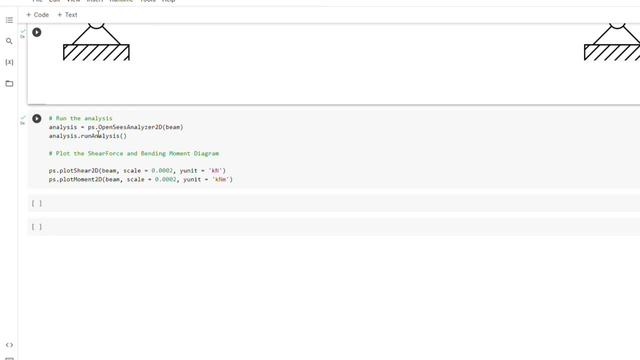 Or the final Thing we are going to do here Is to run the analysis. So we are using the Ps dot openSys analyser 2D And we are passing the beam object Or the beam model Here. So when we run it,